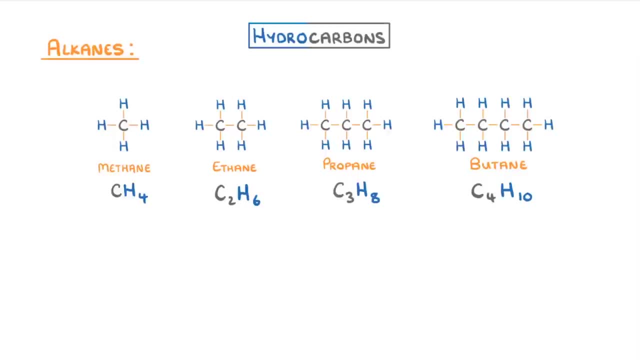 which is C4H10.. Now, if you look at all of these compounds, you'll see that they grow by one carbon and two hydrogens each time, But otherwise they're pretty much the same. We call groups of organic compounds like this homologous series, and it means that they 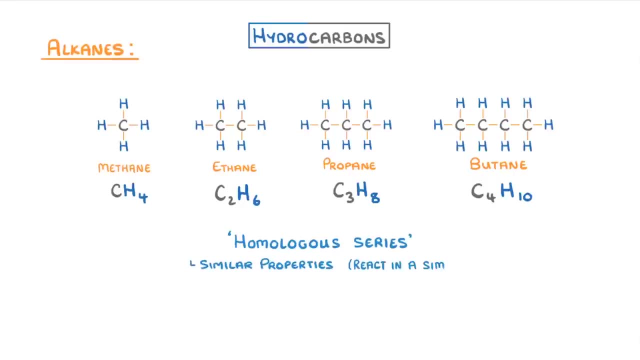 all have similar properties and so react in a similar way. It also means that we can write a general formula which describes the entire series, and in the case of alkanes, the general formula is CnH2n plus 2.. 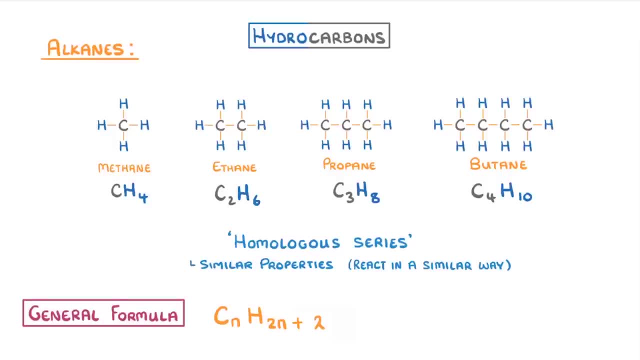 This might look a bit complicated, but all it means is that if the compound contains n carbon atoms, then it will contain two times n plus two more atoms of hydrogen. So if we had an alkane with three carbon atoms, like propane, then n would be three. 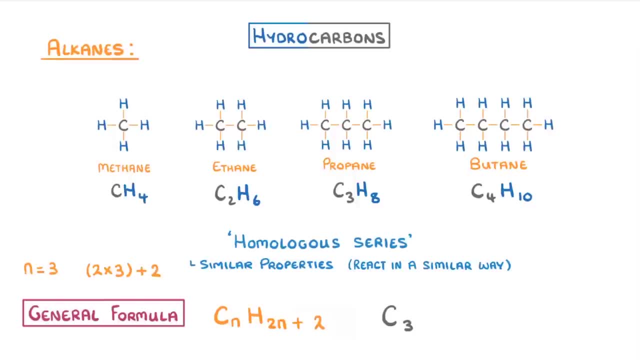 So it would have to have two times three plus two hydrogen atoms, so eight hydrogens, which would give it the formula CnH2n. Now you only need to remember these first four, but you could be asked to use this general formula to work out the molecular formula of much larger ones. 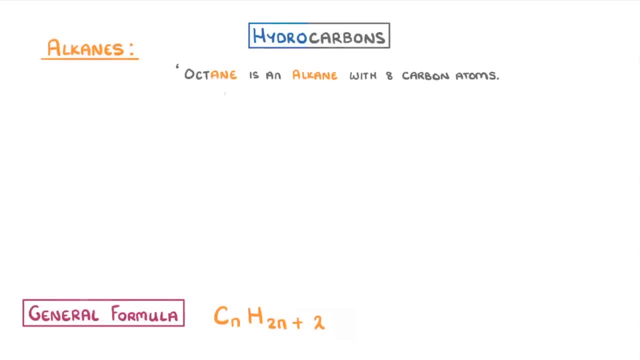 For example, octane is an alkane with eight carbon atoms. What is this molecular formula? Well, we know that for octane, n will be eight, because that's how many carbons it has. So it must have two times eight plus two hydrogens, which gives us sixteen plus two or eighteen. 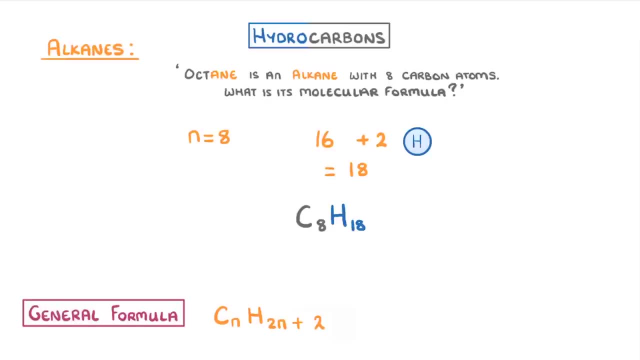 So its molecular formula would be C8H18.. Before we finish, we just need to mention that one of the key features of alkanes is that they're saturated compounds, which means that every carbon atom has four single covalent bonds. 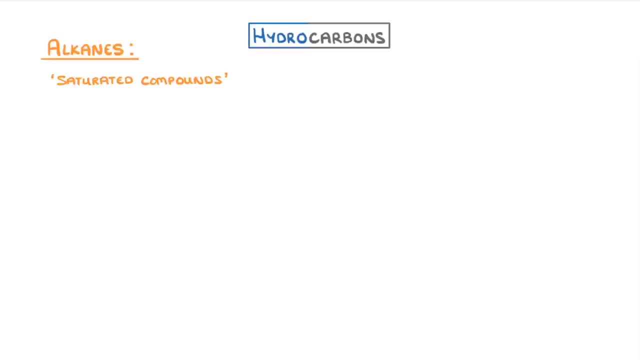 There aren't any double bonds. For example, if we were to take this molecule of propane and change one of these single bonds to a double bond, then each of the carbons involved would have to lose a hydrogen, and what would have left would no longer be an alkane. 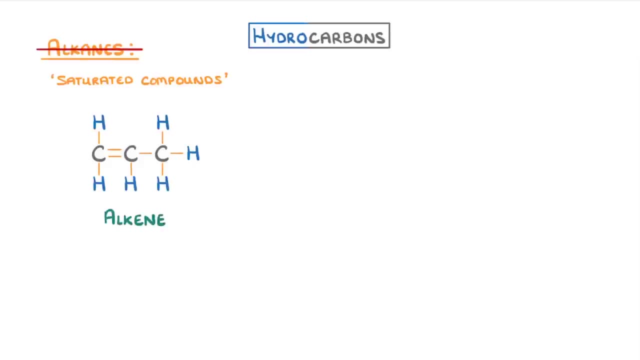 Instead, we would class it as an alkene, which we'll see when we take a look at cracking hydrocarbons in a later video. In our next video, though, we'll stick with alkanes, By taking a look at their properties and seeing how to write equations for their combustion. 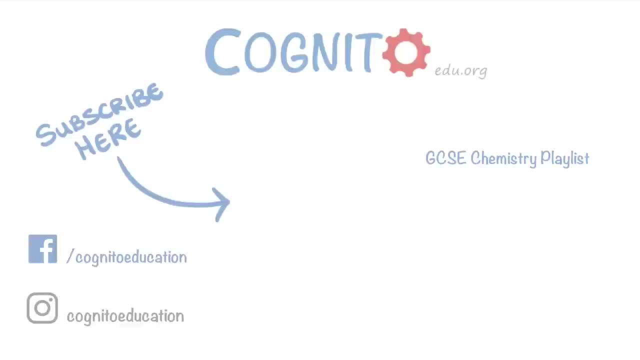 Anyway, that's all for now. So if you enjoyed it, then do tell your friends about us and we'll see you next time. 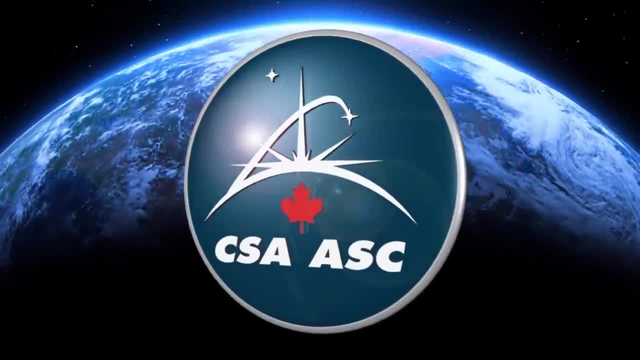 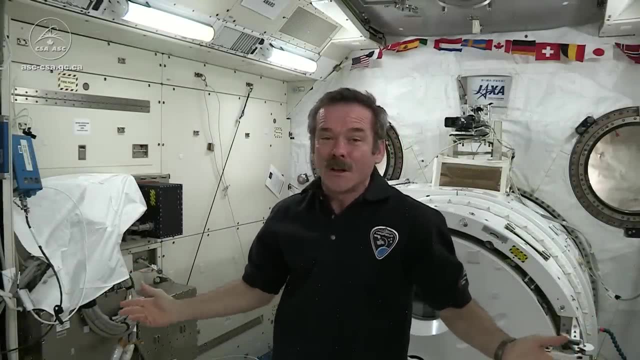 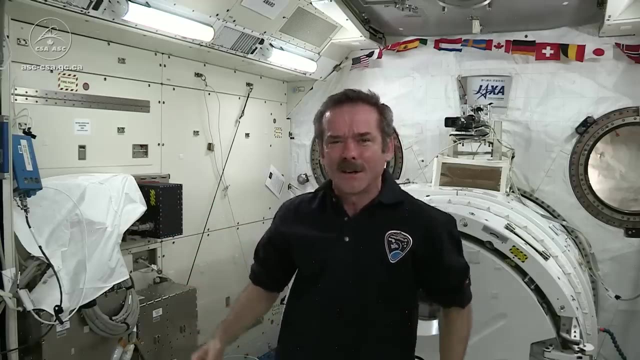 Hi Chris Hadfield, here aboard the International Space Station. We keep busy on board the space station: Long days, lots of work, physical exercise. At the end of it you're tired, but how do you sleep in space In order to make it comfortable for the astronauts? 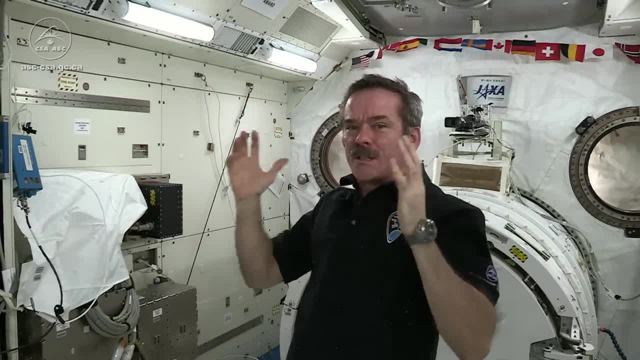 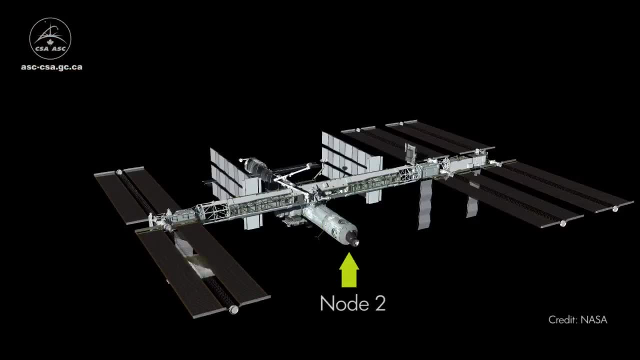 originally they were going to put us all in one habitation module with sleep stations all around it, But the way a station was eventually built. we have sleep stations inside node two, which is in the forward part of the station, and inside the service module, which is in the aft. 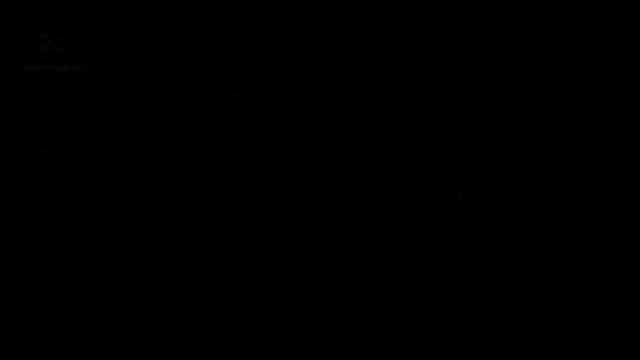 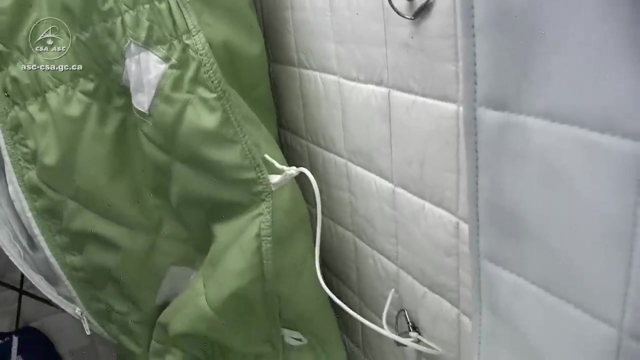 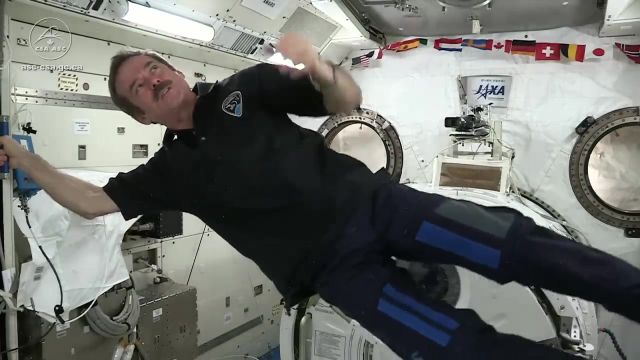 a total of six small bedroom sleep stations or sleep pods, And inside each one is just a sleeping bag tied to the wall. You might think it's uncomfortable not having a mattress and a pillow, but without gravity of course, you don't need anything to hold you up. You can just. 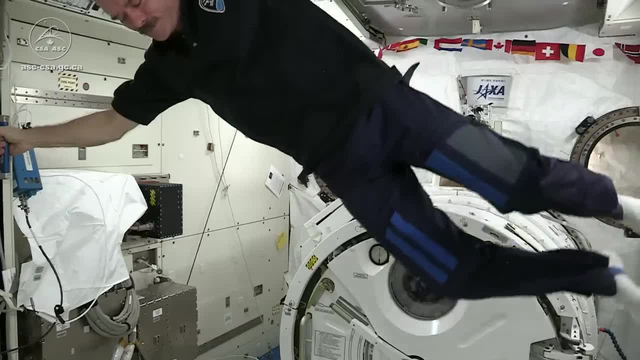 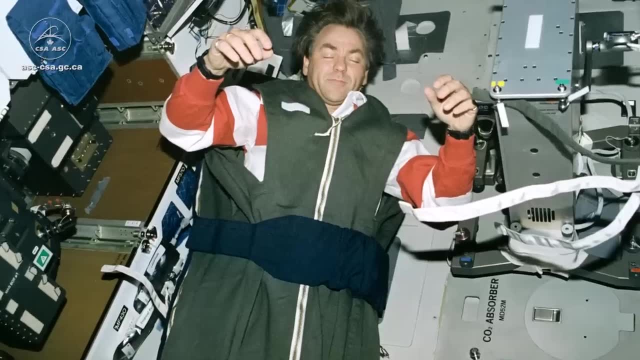 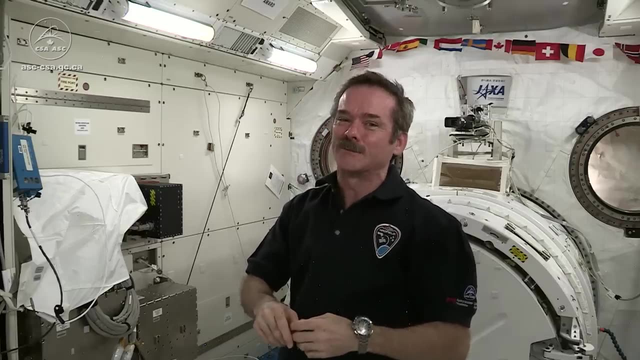 completely relax and you don't even need a pillow in space. You don't even have to hold your head up so you can relax every muscle in your body and your arms float up in front of you. your head tips forward. But before I go to sleep I got to put on my pajamas because I have space jammies. I'll be. 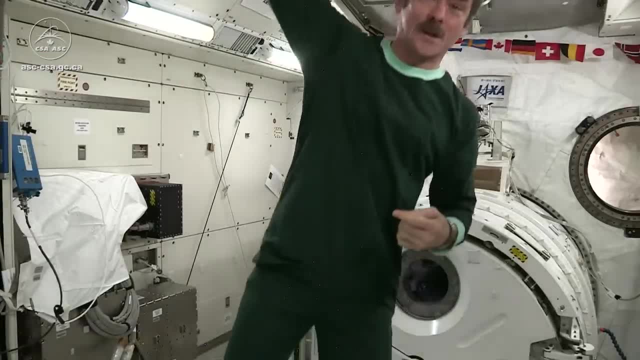 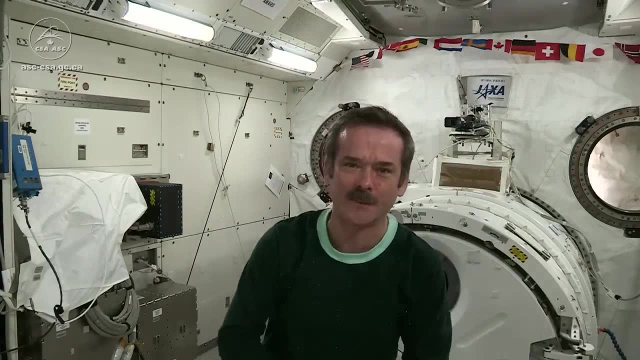